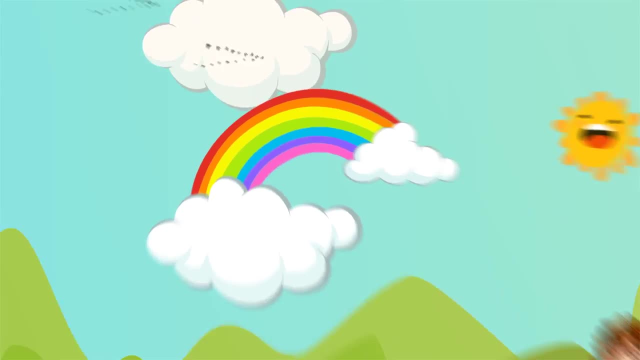 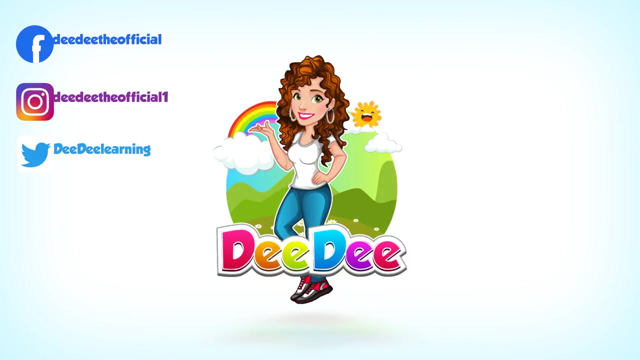 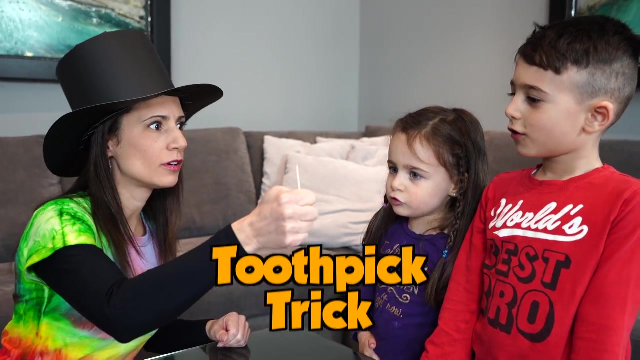 Yeah. So I want to show you my first trick, And it's the toothpick trick. So what do I have in my hands here? Toothpick? Can you feel it? Does it feel It's pinchy on the top right? 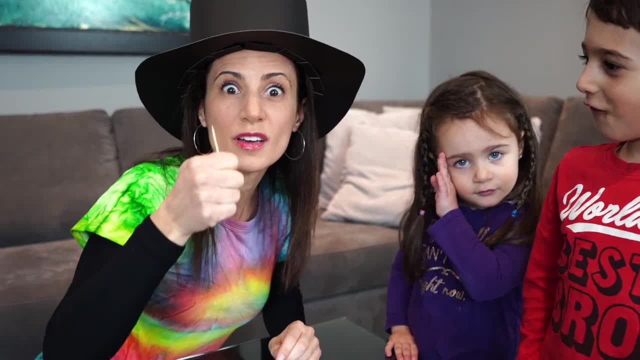 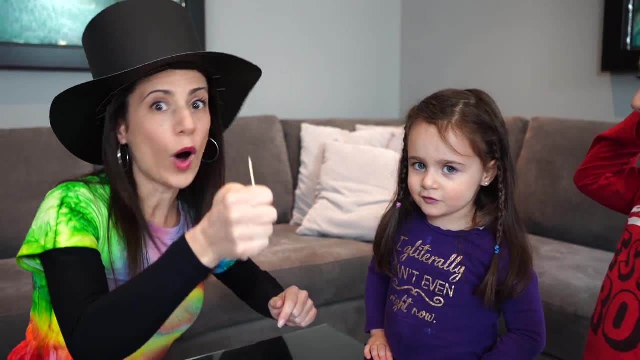 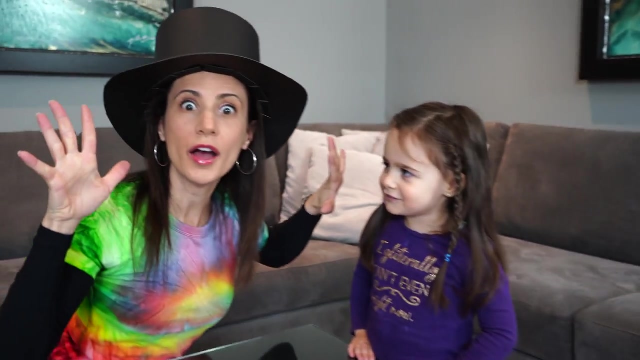 Yeah, Okay, so I'm going to make this toothpick disappear. Are you ready? Are you guys ready? Yeah, Okay, I want you to keep your eye on the toothpick. One, two, three and Whoa, Where'd it go? It's gone, Okay, Hmm, So we lost the toothpick. We need to find it. 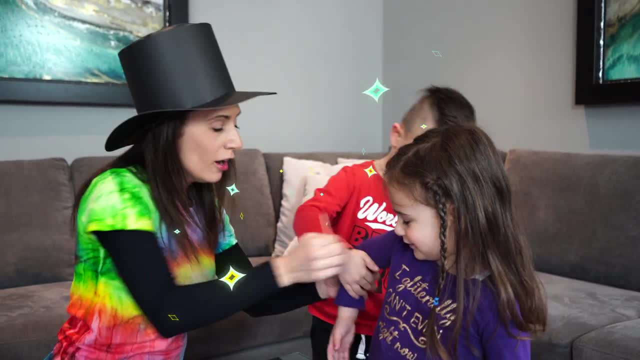 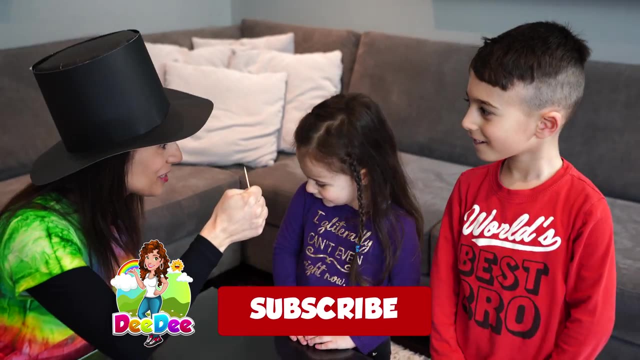 I think it's. Is it under your arm? Let me see. Ah, I got it. It was under her arm. How cool is that? Is that awesome? Yeah, Make sure it's still real. Make sure it's still real. It is right. Do you want to see how it was done? 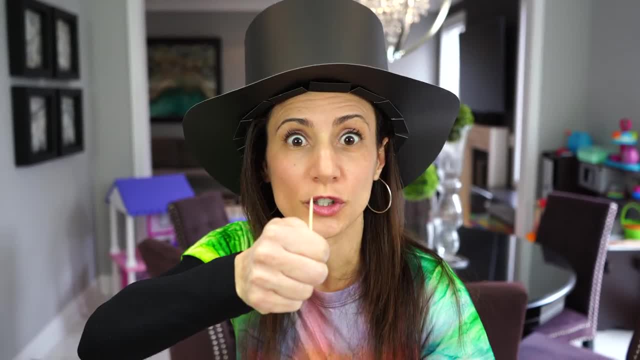 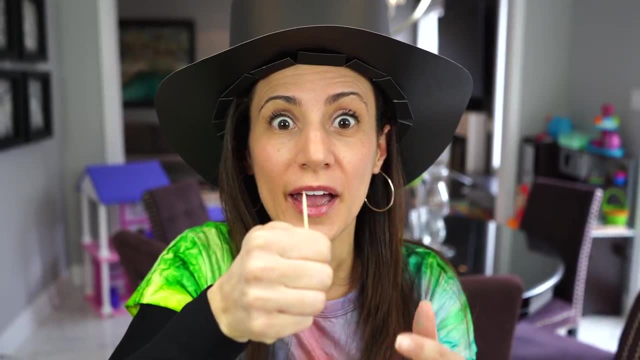 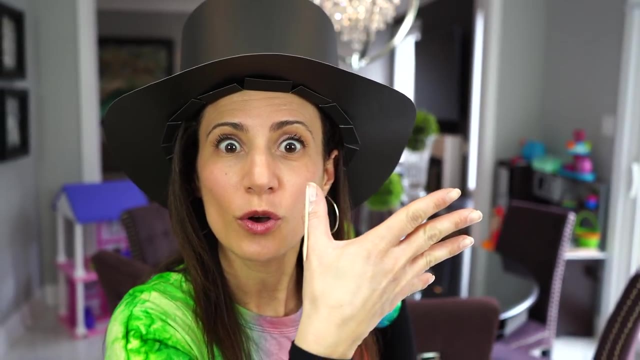 Do you guys want to know how it was done? Yeah, Are you guys ready For the toothpick trick? Did you see that? Let me show you how it works. You need a toothpick and some tape, And what you do is you tape it on your nail like that. So when you close it together and you grab it, there's a toothpick. 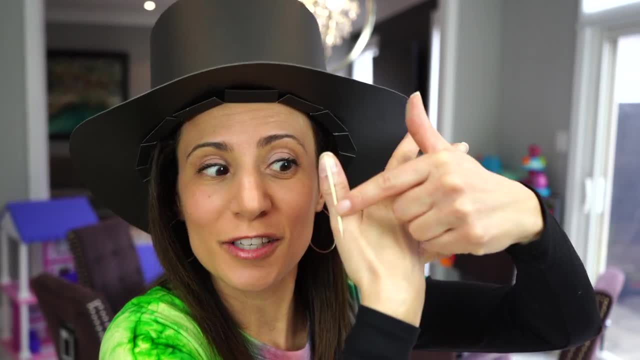 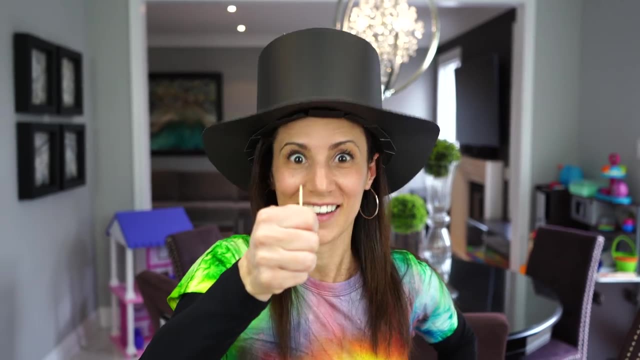 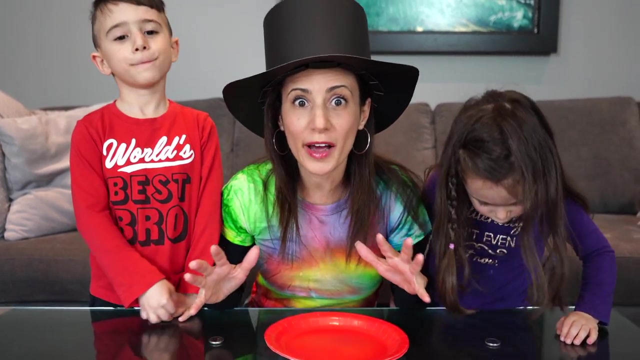 And look at it, It actually hides behind your thumb. That's pretty cool. One more time, Awesome, Awesome. Let's go back and do some more tricks. So for our next trick, we are going to be multiplying money. That's cool, right. 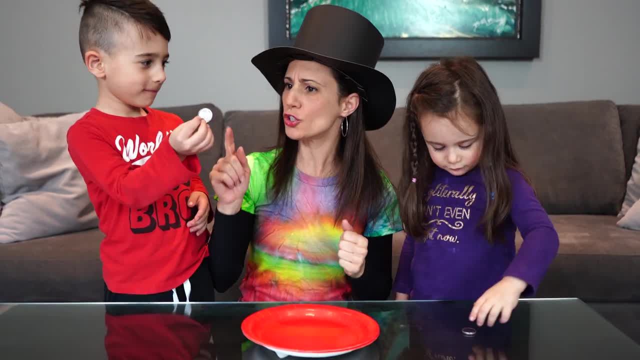 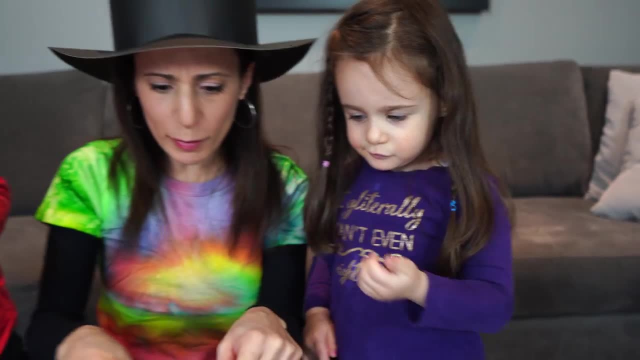 Yeah, Okay. So who has money? Me, Wow, Okay. So you have Quarter- 25 cents, And I have a quarter too, And that's 25 cents, right, Okay? Everybody put their money in. So 25 cents to 25 cents is. 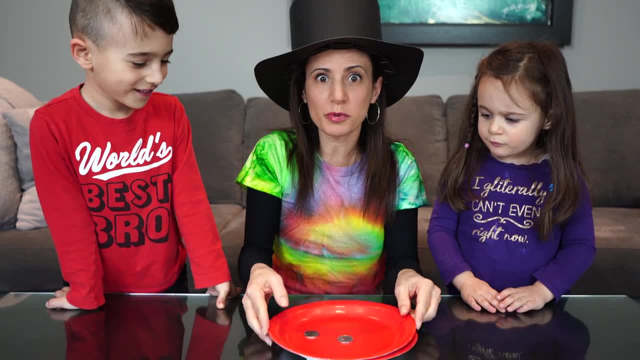 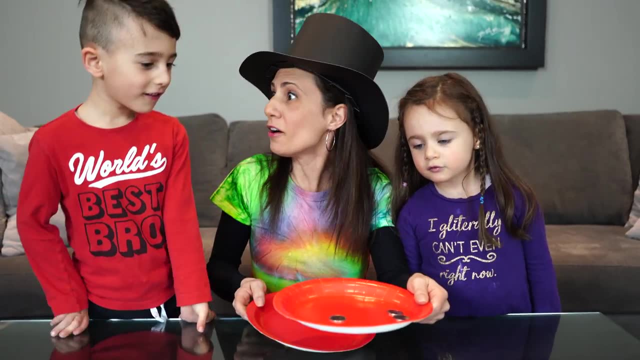 50 cents. You got it. Now we're going to make more money. Ready to multiply, Here we go. Keep an eye on the coins. Keep an eye on the coins. Keep an eye on the coins. And what do we have now? 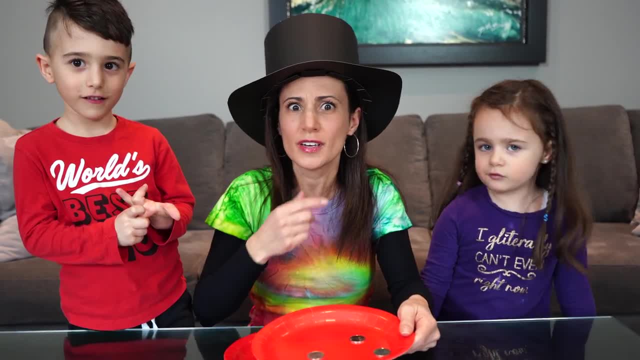 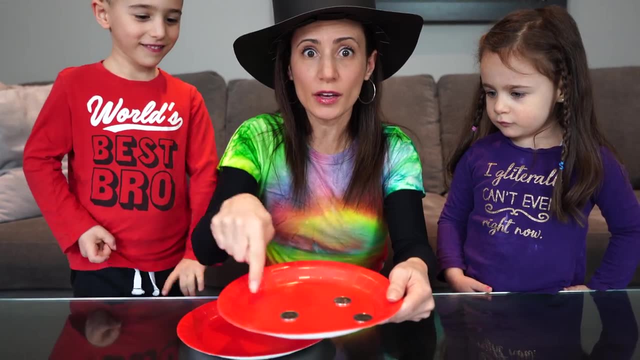 75 cents. Right, because we have three quarters Now. is that enough? No, I think we should add another one, right? Okay, Let's see if we can do it Ready. Keep an eye. We got three, Now we're looking for four, right? 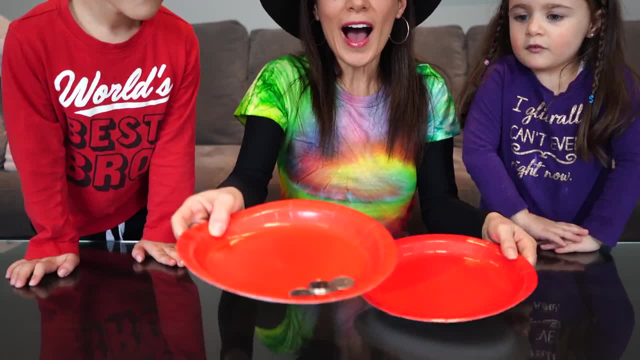 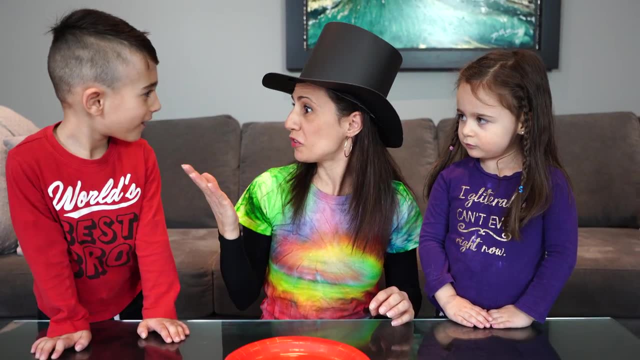 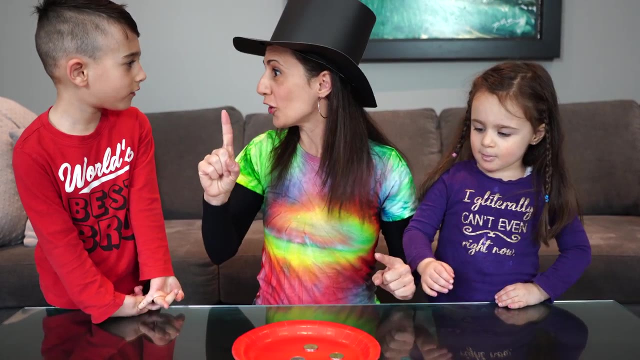 Keep an eye, Keep an eye, Keep an eye And Whoa, Look at that Money, Money. We got four. So we started with 50 cents, Right, And then we got it 75. And now the last one was one dollar. We got a dollar. Cool. Now let me show you how it's done. 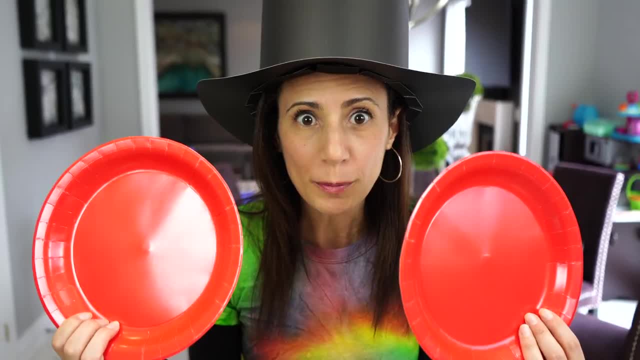 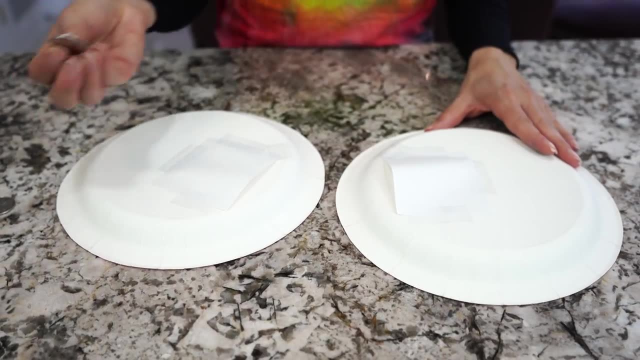 For the multiplying coin trick you need two paper plates, And then we're going to cut out two squares and tape them on three sides of each plate. Then we put our coins in, Slide them in like a little pocket, And then we're ready to flip them over. 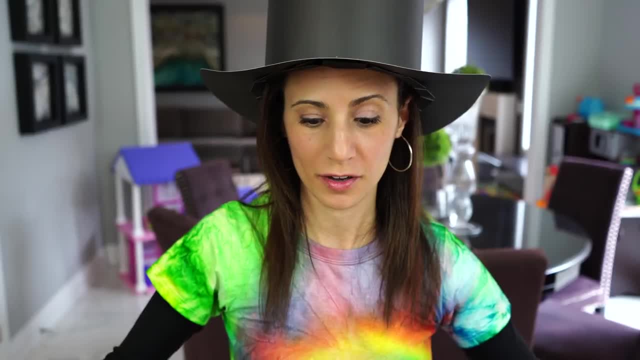 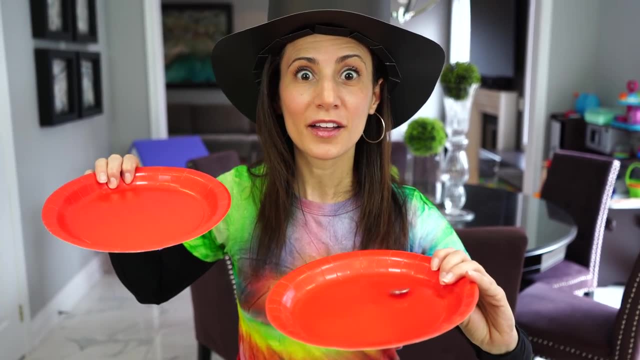 And then we're ready to flip them over, And then we're ready to flip them over. So you can't see the coins yet. But when you shuffle them over, one over another, there's one coin And then you do the other one. 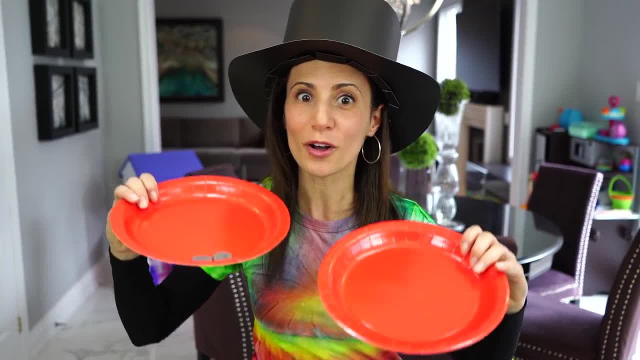 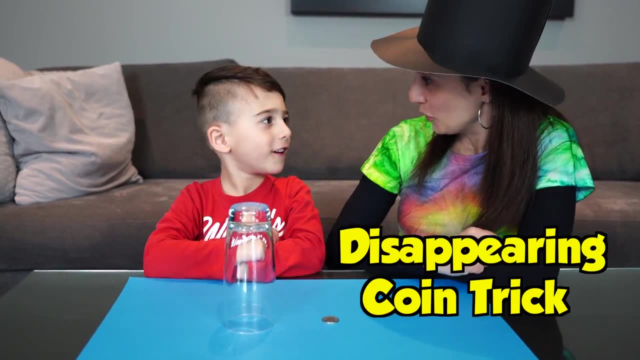 And you get two coins. And that's how you do the multiplying coin trick. Let's do another one. Hey guys, I have a trick for you. You do Yes. So what is it? So I have a glass and I'm going to cover up the coin. 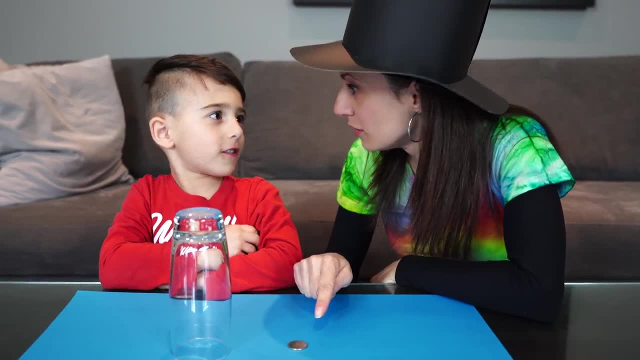 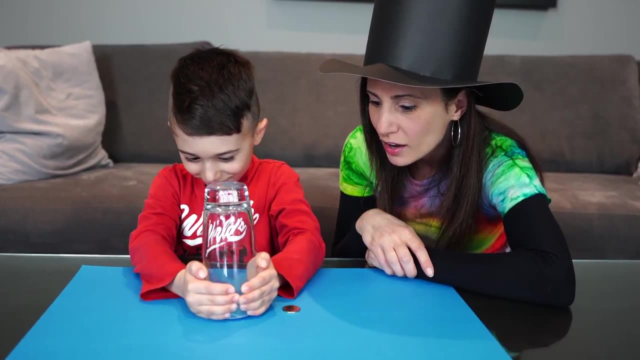 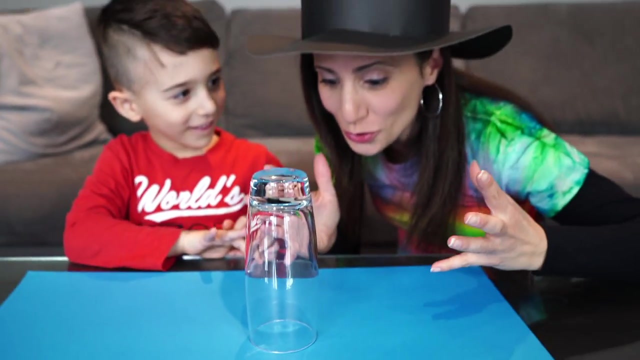 So you're going to make this coin disappear? Yes, Wow, I can't wait to see this. Okay, Let's see it. Mateo, Wow, It's gone. How did you do that? Okay, So you made it disappear. Can you actually bring it back? 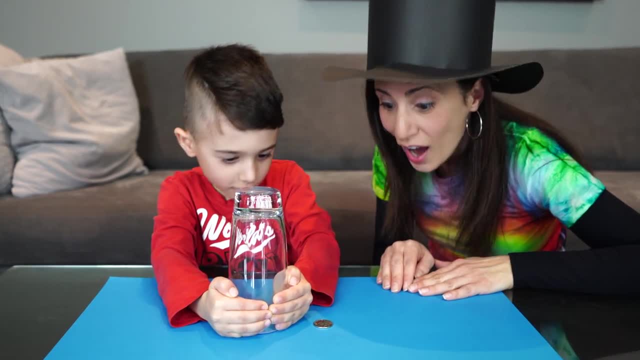 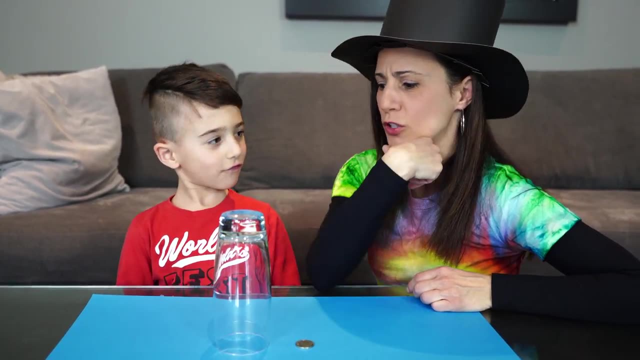 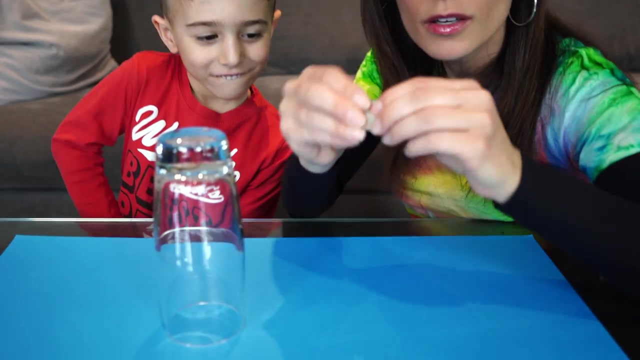 Yeah, You can. Okay, Wow, It came back. Wow, That's awesome. Now there must be something tricky about this. Can I check the coin? Yeah, Okay, So the coin, it's actually real. It doesn't bend And it's not those chocolate ones, is it? 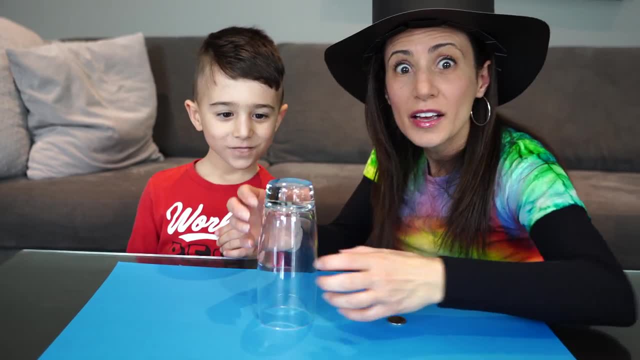 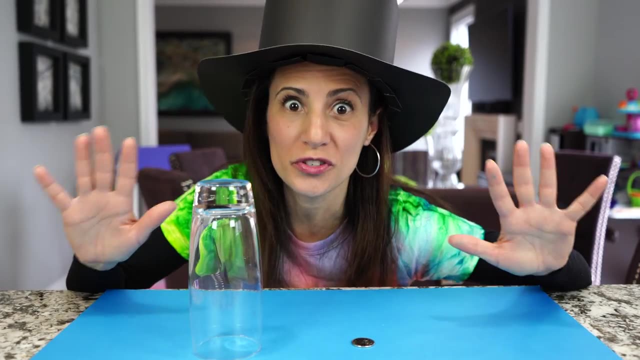 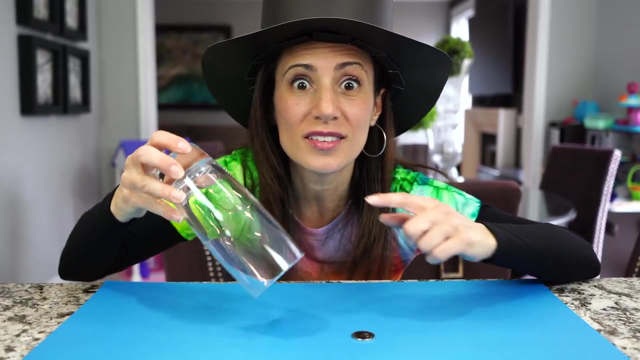 No, No, And the glass. it's a real glass. Hmm, For the disappearing coin trick. with the glass it's super simple. So you need a colorful piece of paper And what you're going to do is you're going to trace a circle that's the same rim of your glass. 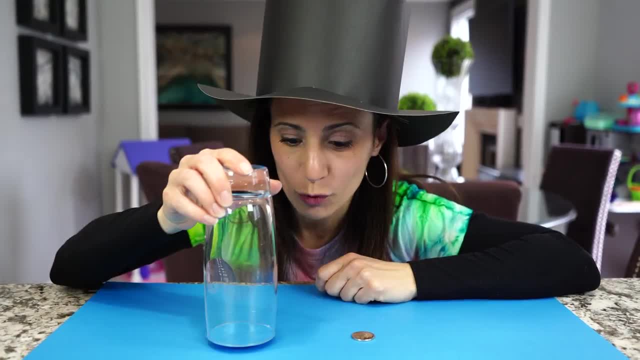 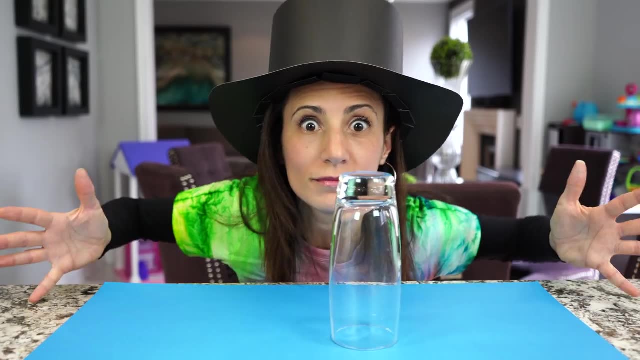 And you're going to glue it on like that. So when we do the trick, you cover the glass with your fingers and you move it over the coin. Now look, It's gone. We hid it And it's actually under there. See, Pretty cool. 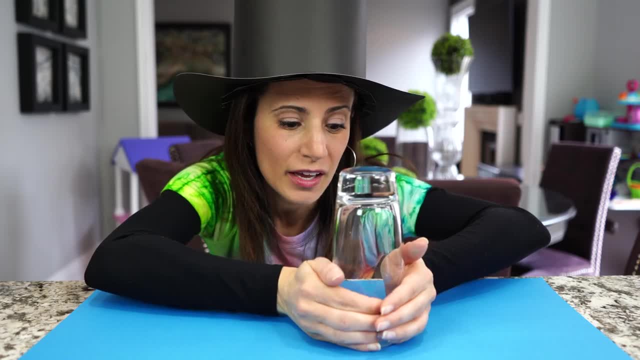 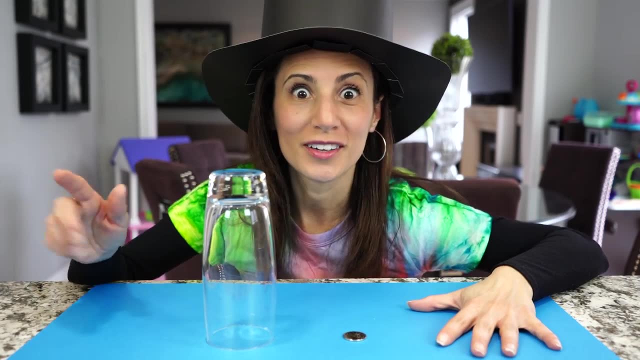 Then, when you bring it back, you cover your hands again And you bring it back And voila, There's the coin. That's the disappearing coin trick. Pretty easy For the next magic trick. I need your help, Mikhail. 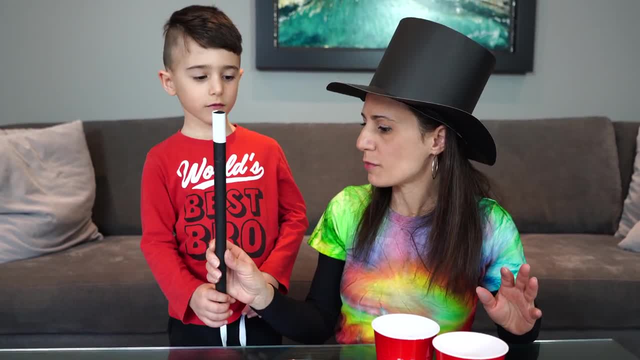 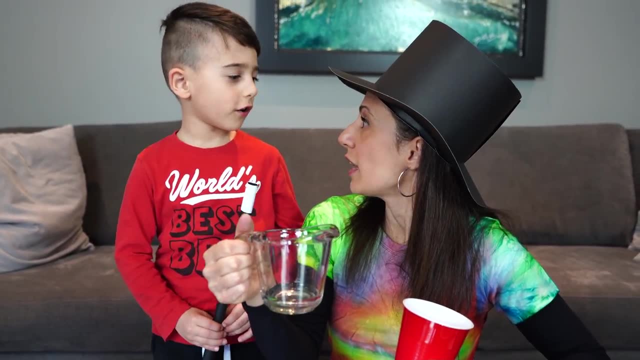 Okay, Okay, So can you hold this for me? the magic wand. Yeah, All right, Now we're going to start off with some water. Now, do you have a favorite color? Blue, It's blue. Okay, So we're going to try to change this water into blue water, Got it? 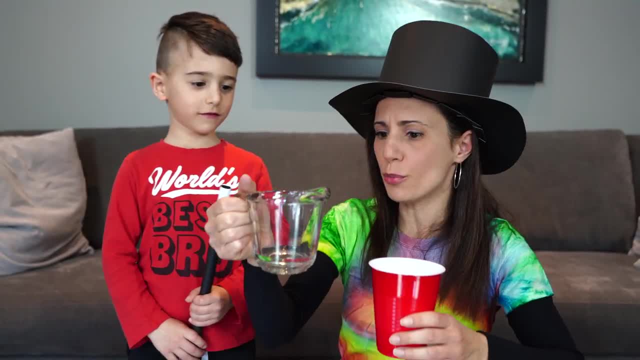 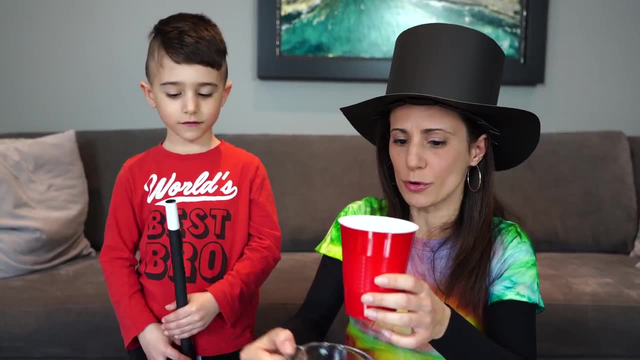 Yeah, And you're going to help me with that magic wand, So I'm going to pour it in And then we are going to do abracadabra on top and say: change this water blue. Can you do that for me? 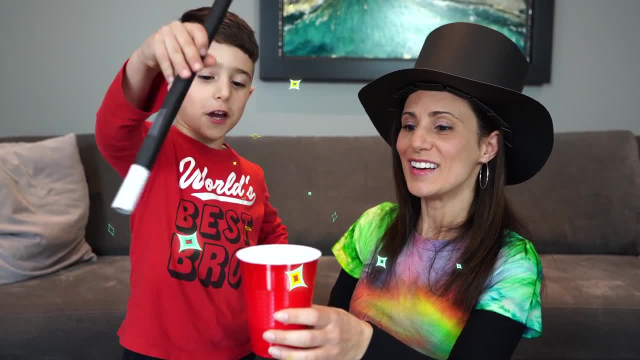 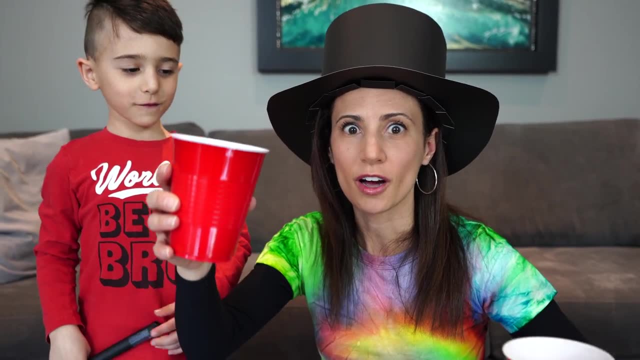 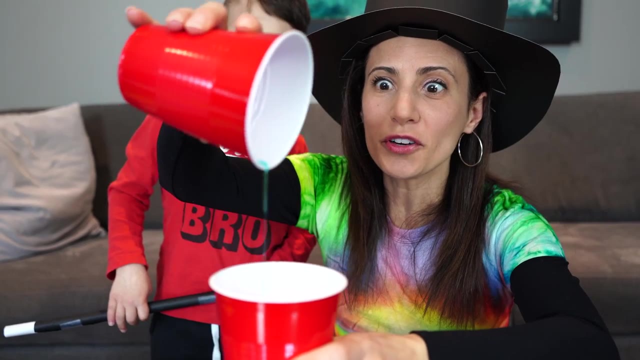 Yeah, Okay, Go Abracadabra, Change this water blue. You think it worked? Yeah, Let's see if your magic and the magic wand helped. Are you ready? Let's see if Mikhail was right. See the color. You did turn it blue. 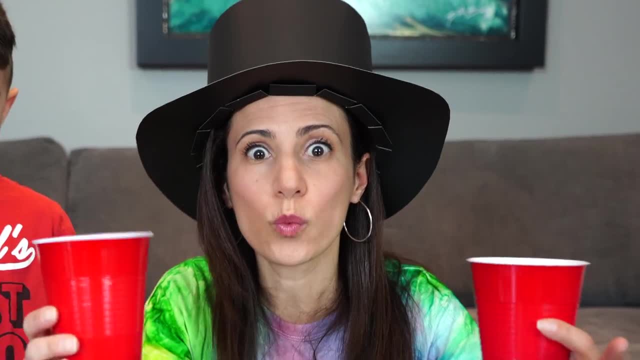 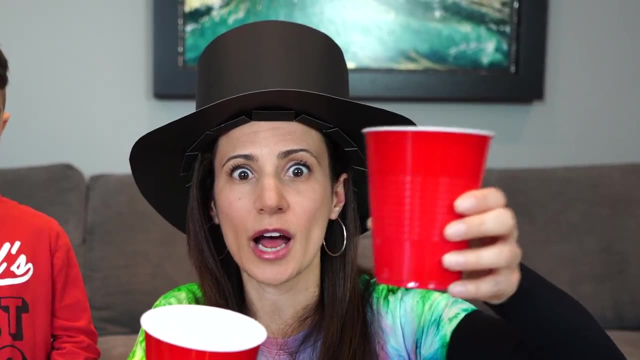 Cool, That was cool. So we turned the water into blue water, right Yeah, And we poured it in here. So now there's blue water in here, Let's pour it back out and see what happened. But I think maybe we should abracadabra and see if we can make the actual water disappear. 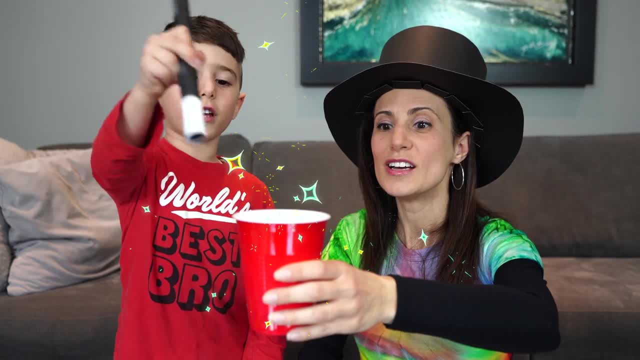 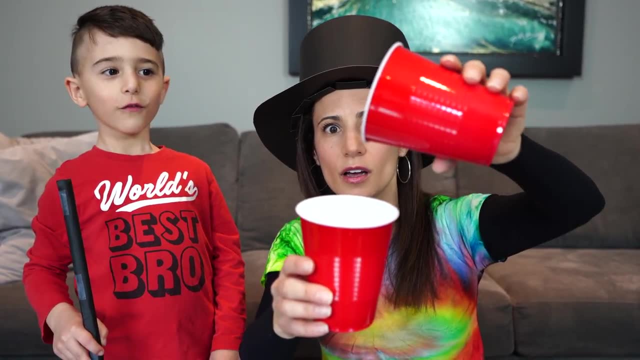 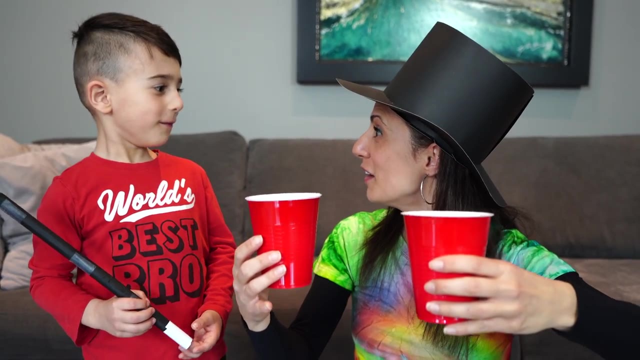 Can you do that for me? Yeah, Okay, Let's see Abracadabra Make the water disappear. Whoa, I wonder if it worked. Are you ready? And Mateo, you made the water disappear. That was so cool. Do you want to know how you do it? 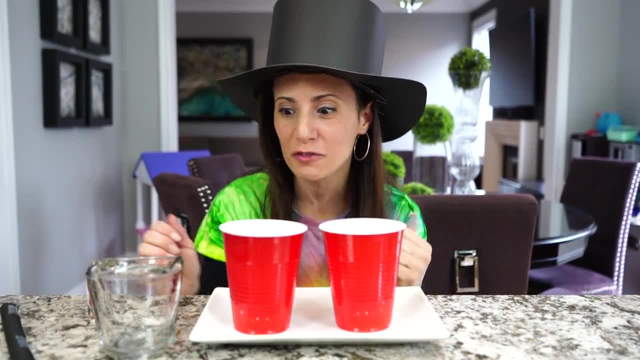 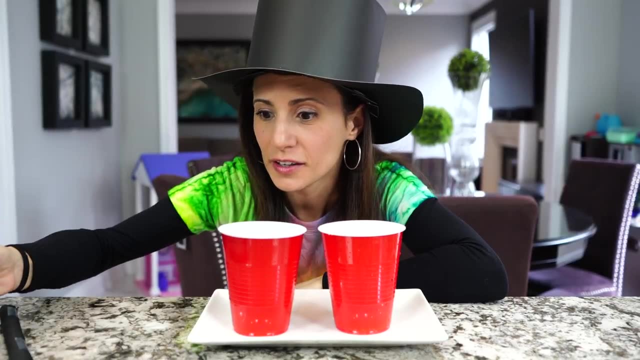 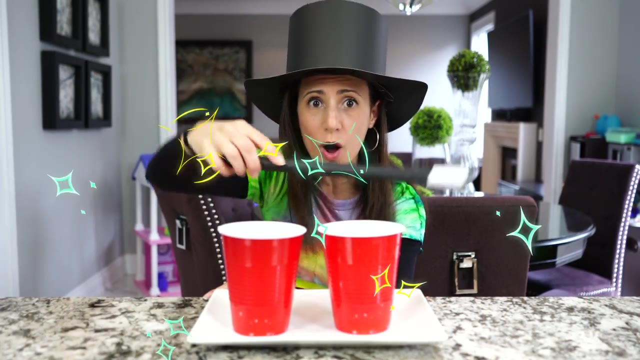 Yeah, Okay, Let's do this one one more time. It's my favorite, So we're going to change our water to a different color. Ready, My special wand. Hocus Pocus, Alamodocus, Make my water blue. 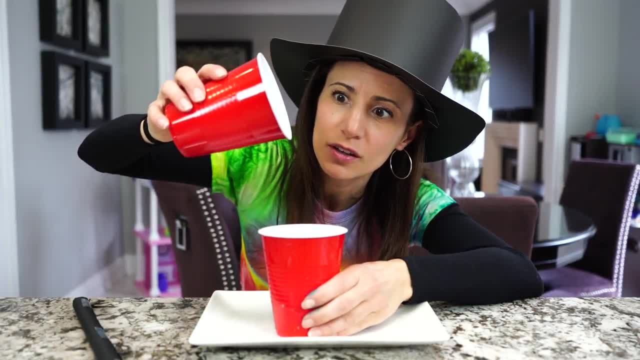 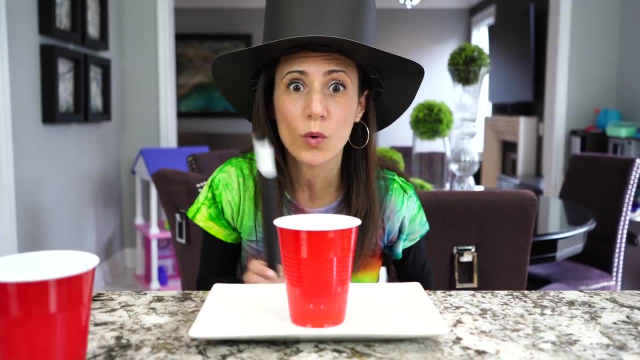 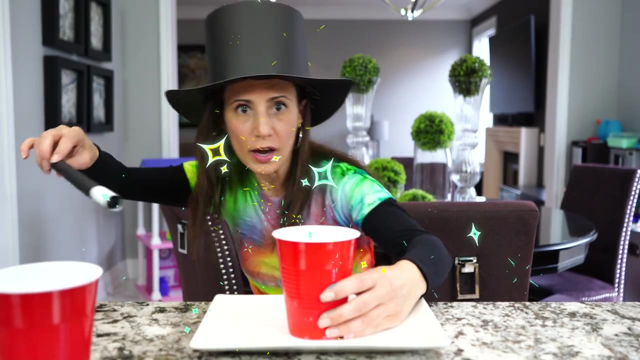 Let's see what happened. Did it change? My water is blue. It worked, Okay, So we made the water blue, But let's make our blue water disappear. So abracadabra, Abracadabra, Make my blue water disappear. 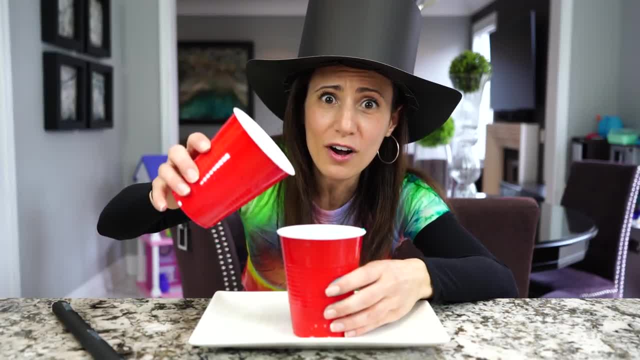 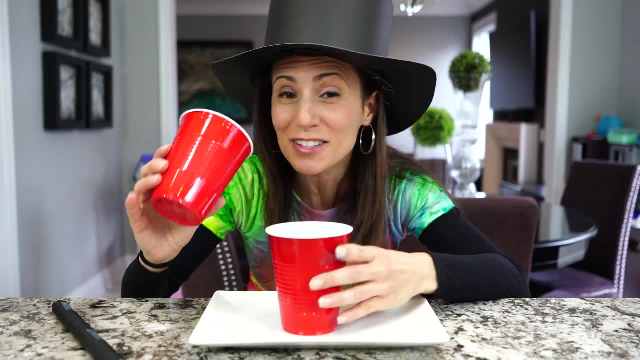 Let's see what happens. Ready, Here we go. Where did the water go? It disappeared. It's gone. That's so awesome. Now let me tell you the trick to this. So we're going to add our regular water in here. 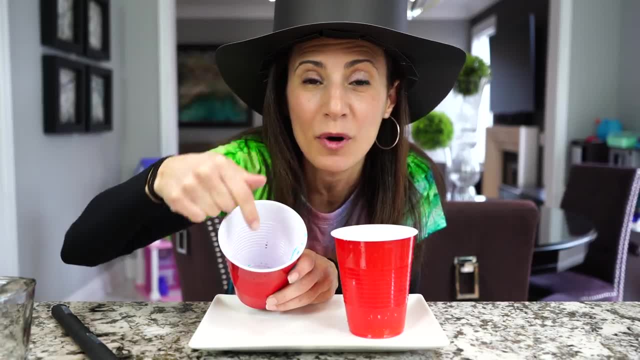 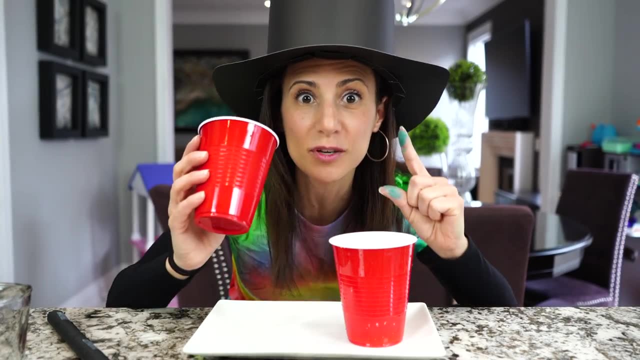 But when you pour it in here, there's actually a dab of food coloring. So pick any color you like. Then, when you change it into the color and you pour it into this cup to disappear, look what's inside the cup. 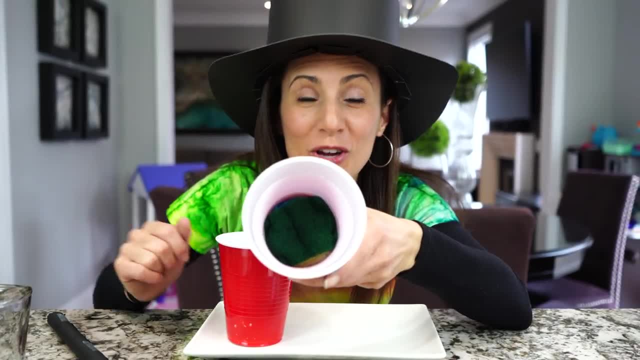 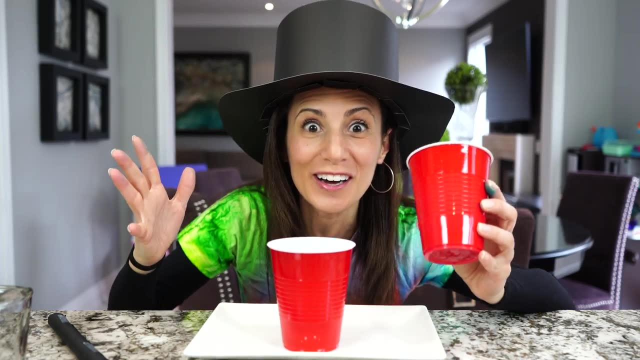 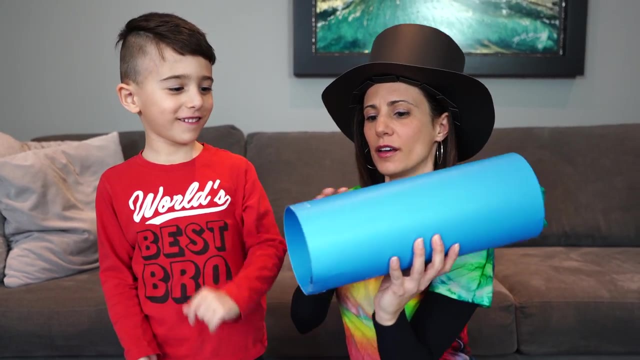 Actually a sponge, So all the water is going to absorb into the sponge and then you have no water left. Cool, For the last trick, Mateo, we have a tube here. See that? Yeah, Feel it. Okay, Can we see inside right through? I can see, Can I see you? You got it right. 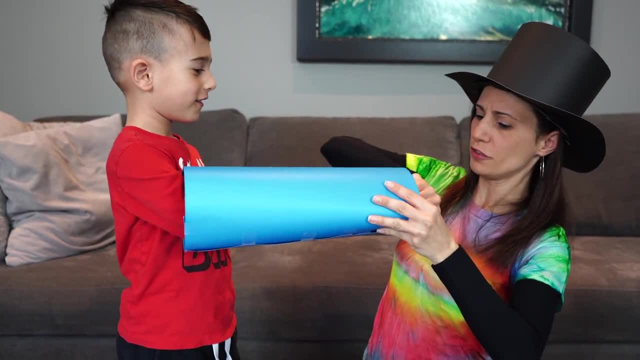 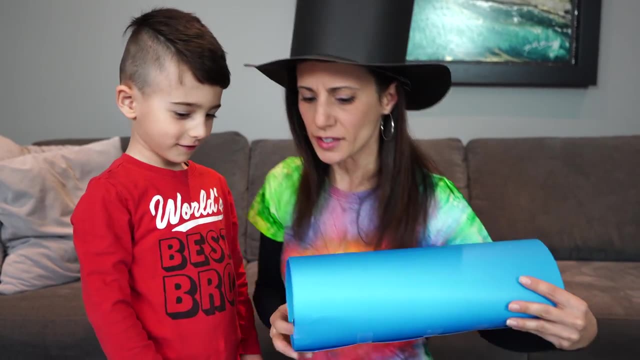 Yeah, Now can you put your hand through and make sure it's real? Yeah, All the way through. Can you feel it? Oh, yeah, I see your fingers. Okay, So that's good. Now I need you to grab the magic wand again for me, and I want you to do Hocus Pocus and maybe we can have something come out of here. 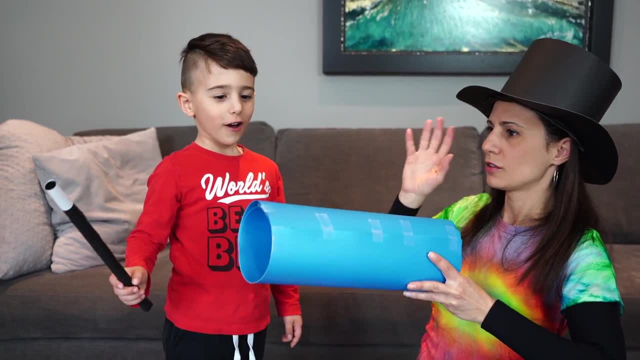 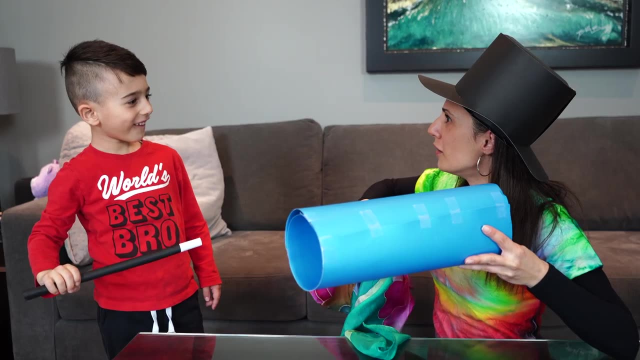 Okay, What do you think? Yeah, Yeah, Okay, Ready Go, Hocus, Pocus, Whoa, Did you see that? Where did that come from? Where did it come from? I don't know, You don't know, But it's still empty. Can you put your arm through? 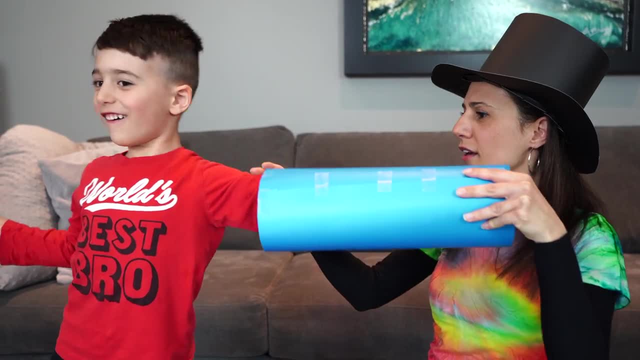 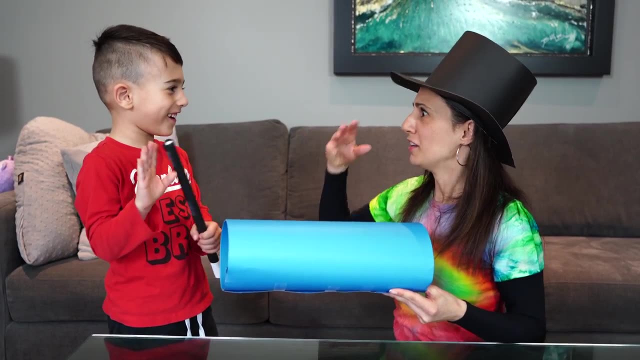 Yeah, There's nothing inside, is there? Look Okay. Hmm, So we got that one out. Do you think there's anything else that we can maybe come out of here? Yeah, You do. We want to try one more time.